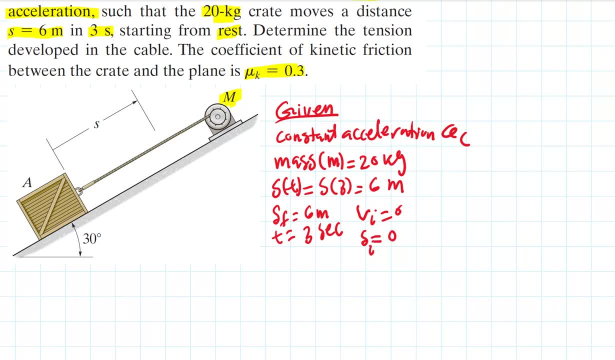 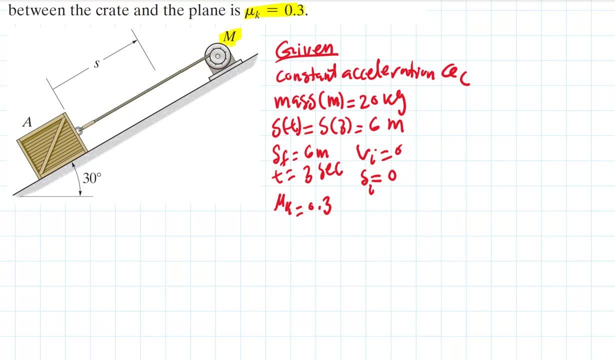 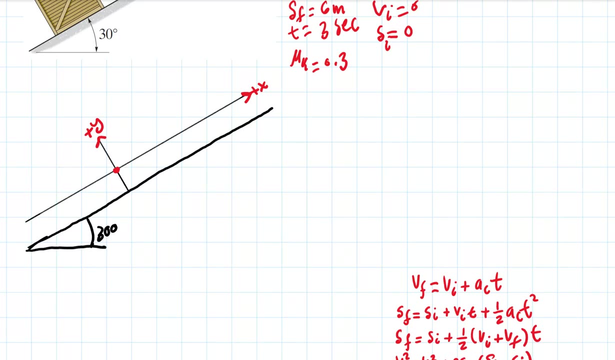 And the coefficient between the crate and the plane is 0.3.. So that tells us there is a friction between them. So we need to account for friction. Alright, So here what we will do is we will draw the free body diagram. 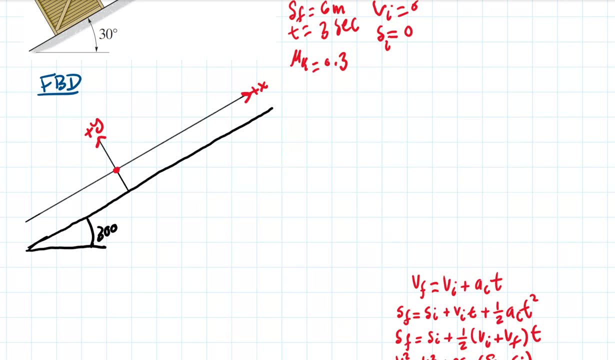 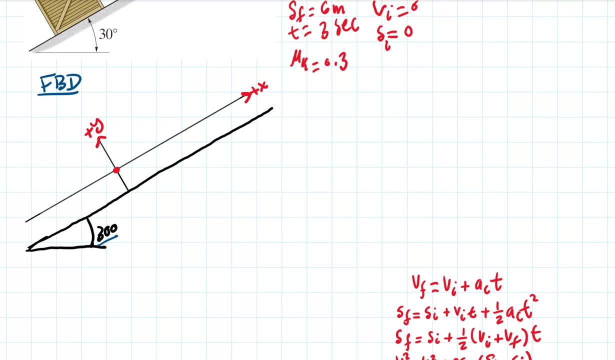 gravity of this crate as a particle. so first thing we want to count for is the mass times gravity, and we can add the mass times gravity into two component, its vertical component and its horizontal component. and this angle is theta, just like this one, 30 degree, so this is 30 degree. 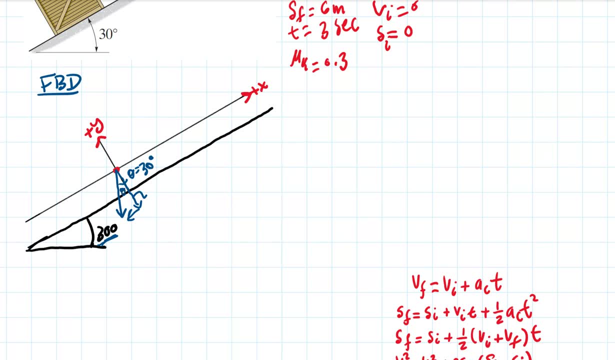 this right here. since it's adjacent to the angle, theta, so it will be mass times, gravity cosine theta. and since this is opposite to the angle, so it will be mass times, gravity times sine theta, and this will be your mass times gravity. and since the crate is on the plane, the. 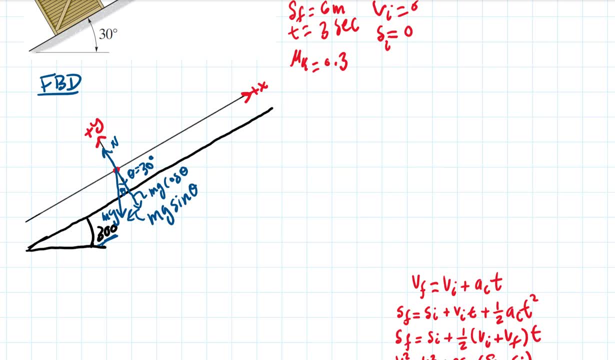 surface plane will apply and will generate a force or a neutral force on the crate. we are told that we have a friction coefficient, so that mean and, and, and we know that the, the particle is moving to the, to the right up, so the friction will oppose the movement. and here 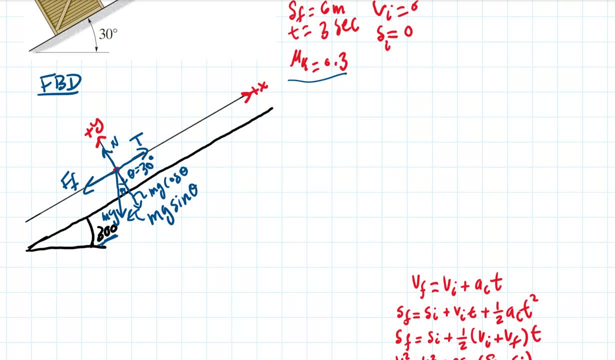 the tension in the cable is the force that is used to pull the crate up the hill or up this incline. so next, what we will do is we want to sum the forces in the y direction and the sum the forces in the x direction. summing the forces in the y direction as: 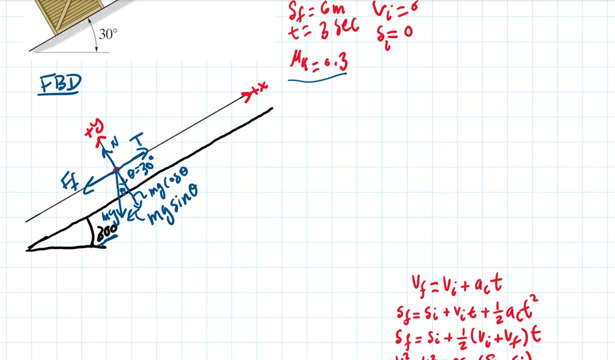 we can see there is no movement in the y direction. so let's do that. so here, oh, going up- is positive sum of the forces in the y direction equal to zero. so the we have n, and then we have minus mass times, gravity times, cosine, theta, equal to zero. 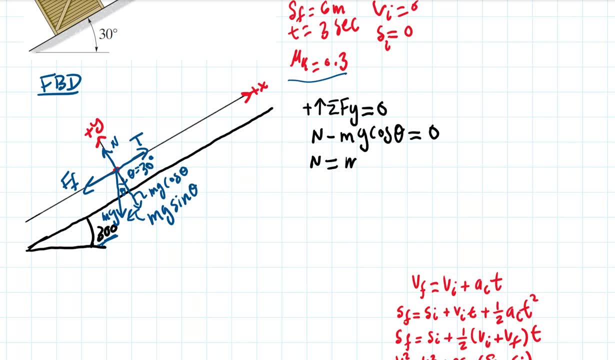 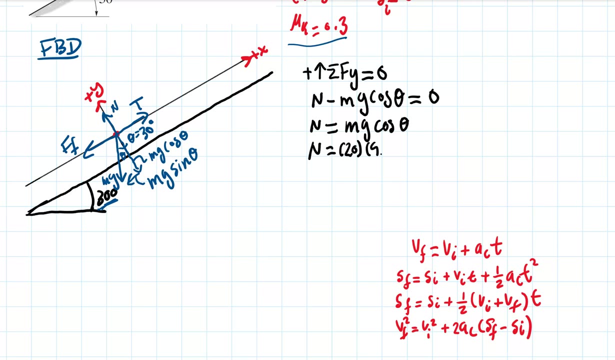 so now to n and move to the other side: mass times, gravity times cosine, theta. so n will equal to what the mass is given to us as 20 kilogram and the gravity is 9.81 times cosine 30 degree. so let's so 20 times 9.81. 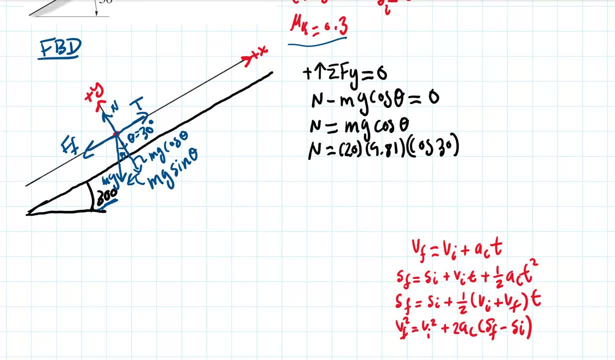 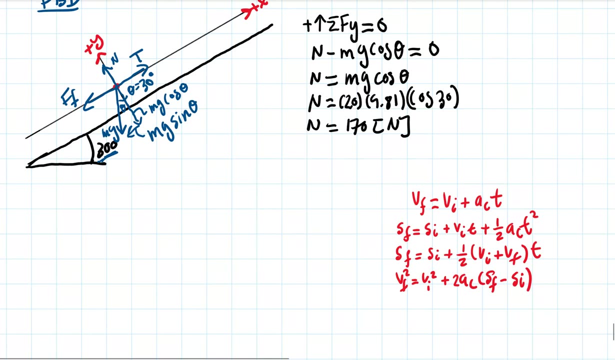 times cosine 30. so it gives me 169.9. so i'm just going to say 170.. all right, so now we there is a relationship between the normal force and friction, because force due to friction is equal to mu k times m. so 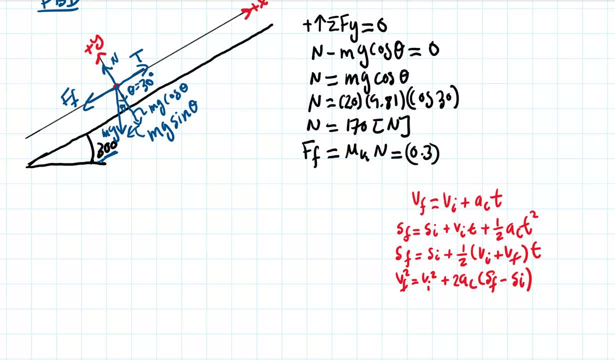 Mu K is given to us as 0.3 times and the normal, we found it to be 170.. So that will equal to what? So we said: 170 times 0.3 gives me 51 newton. All right, so now, next we will add up the external forces applied on the mass in the X direction. 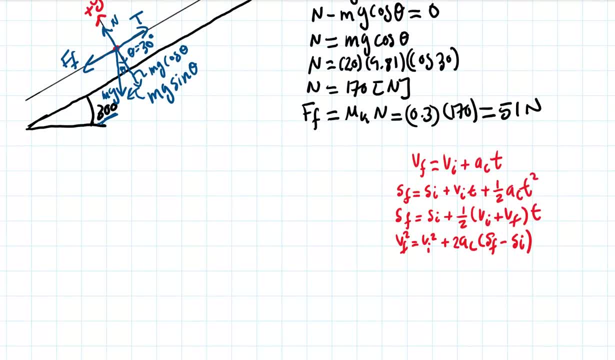 So here on the side, plus sum of the forces in the X direction equal to mass times, acceleration in the X direction. So going to the right is positive. So here we have the tension in the cable that is pulling, the crate, minus the mass times, the gravity. 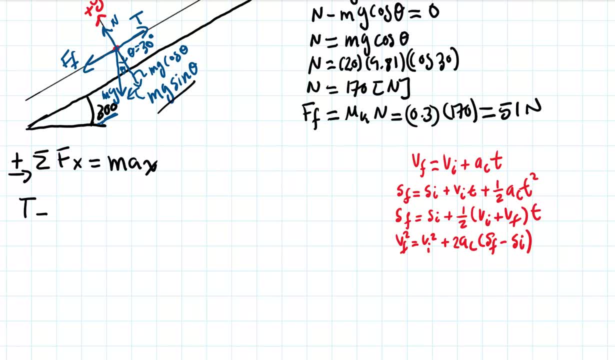 the horizontal component of the weight of the crate, mass, times times, gravity times, sine theta and the force of the friction. we found it to be 51 newton, equal to the mass of the crate we said is 20, acceleration in the X direction. 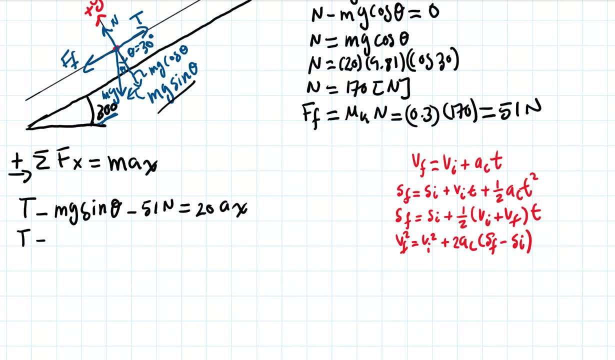 We can simplify this more so we know that mass here is 20.. This is 9.81, and this is sine 30. So let's plug this into our calculator. So it's 20 times 9.81, times sine 30, it will give us 98.1.. 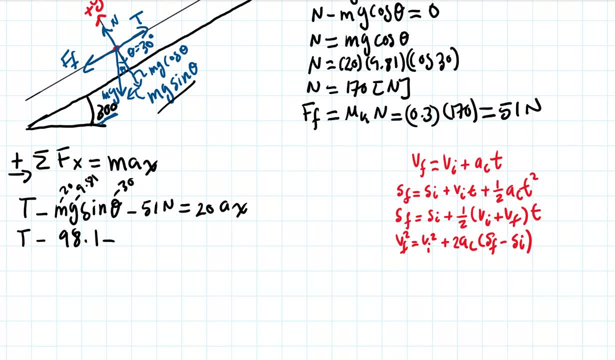 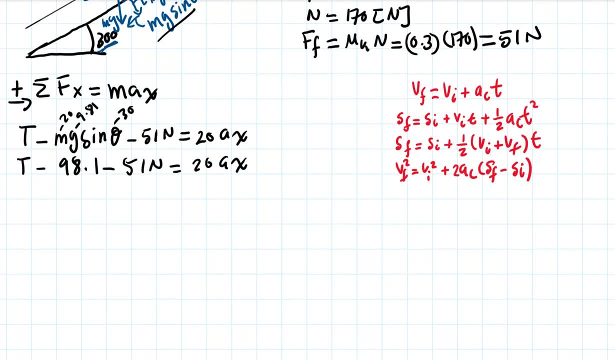 98.1 minus 51 newton, equal to 20 AX. We can simplify it more. T will be minus 98.1 minus 51. It will give us minus 140.. So make that 9.1 times 9.1 into 8.. 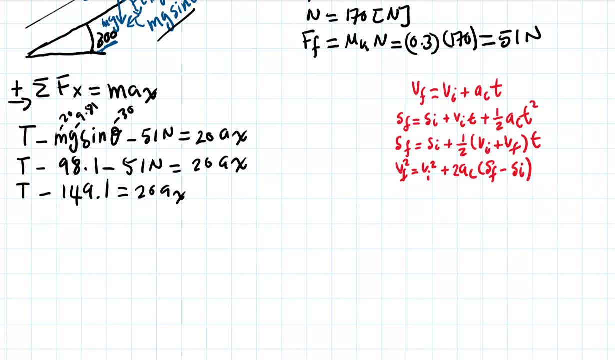 9.1 equals to 20 AX. All right, So right here, what is our goal? Our goal here is to find what is T, But here we cannot find AX. So acceleration equal constant. then we can use these equations right here. these are: 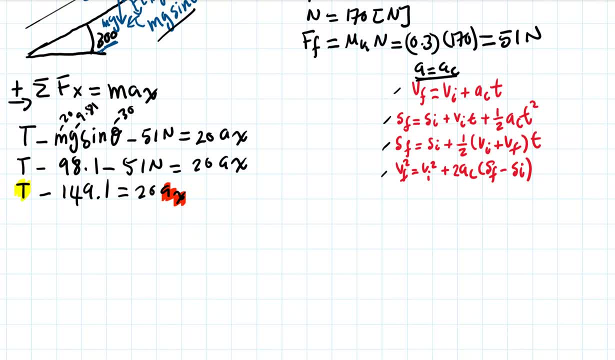 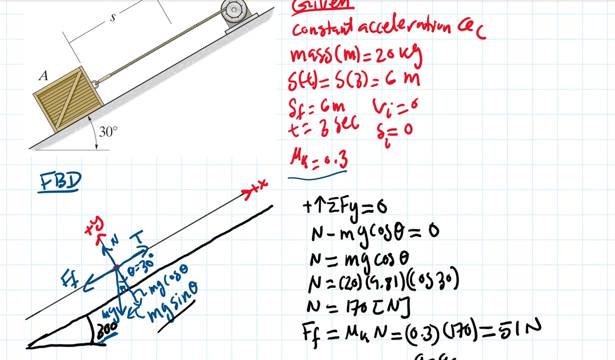 constant acceleration equations, so we can use these equations to find our acceleration in the x-direction. so let's so? what do we? so? what do we have? so from what is given to us? that the final position is 6, the initial acceleration is initial, velocity is 0, initial position is 0 and time is 3 seconds. okay, 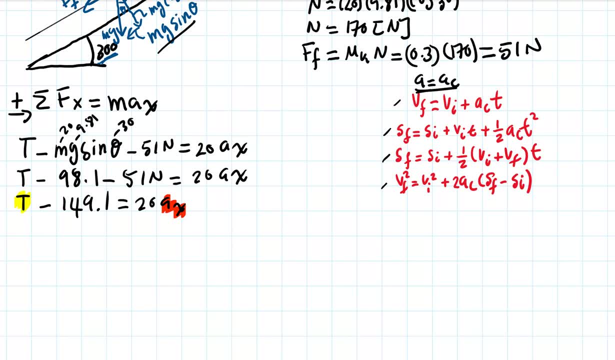 so let's let's take a look at the first equation and see if it works. so here it deals with final velocity. we don't have final velocity, so the first one won't work. let's take a look at the second one. the second one we have, we have the final. 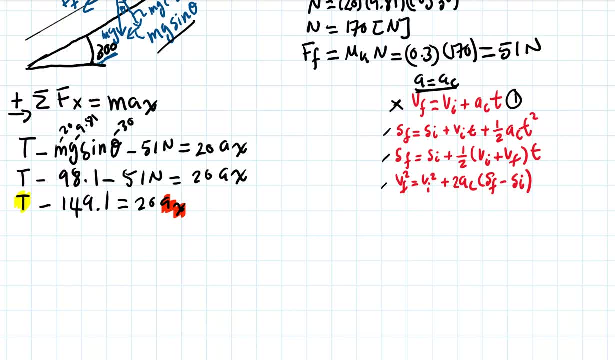 which is 6 meters, initial is 0, the V initial is also 0 and 1 half and t is 3 seconds. so we can use this equation to solve for acceleration. but let's take a look at the third and the fourth one. the third one also. 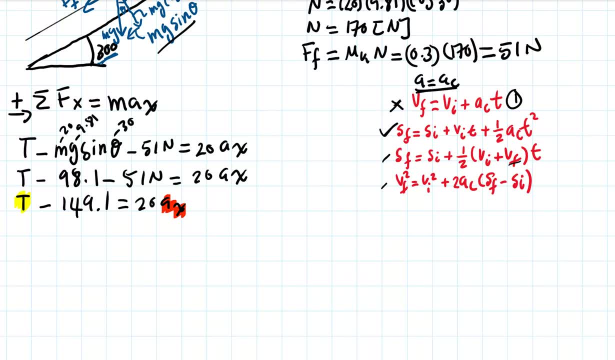 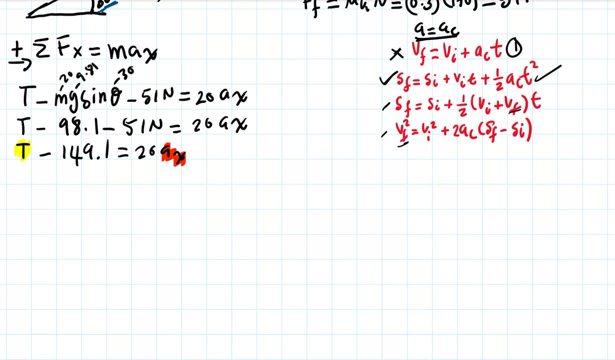 involves final velocity. we don't have it. and the fourth one also involves the final velocity, which we don't have it. so the best fit is to use the second equation. so the second equation is the correct one to use, so let's plug in the given values that we have. so the s final. 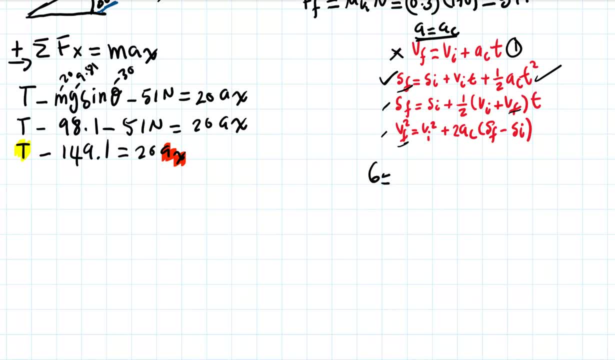 is 6 meters, that equals the S initial 0, and the initial velocity is also 0, 0 times time is 0 plus 1, half a constant, and the time here we said is 3 squared. so six equals it with one half. so then i'll give you. 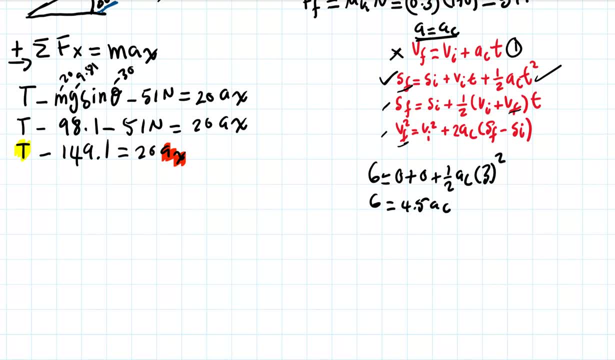 four point five a sub c. so a sub c will equal to six divided by four point half. so accelerated constant. si. cdcd, os��, diBooks y 45, Kristin C Writing b Jack position table lipstick ink- Yeon paisley. фотограф Mutter photoizz. 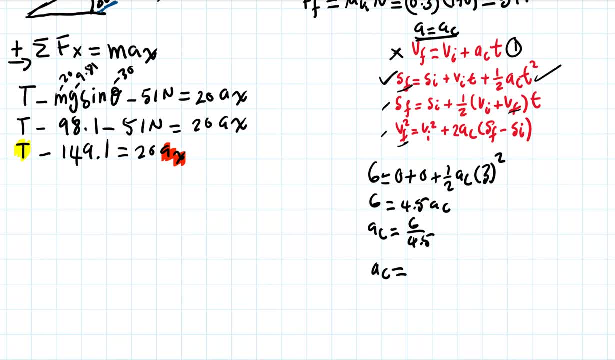 acceleration, constant acceleration will be. so 6 divided by 4.5 is 1.33, so this will be 1.33 meter per second squared. so now what we can do is we can take this constant acceleration and plug it in here, and that should give us the tension. 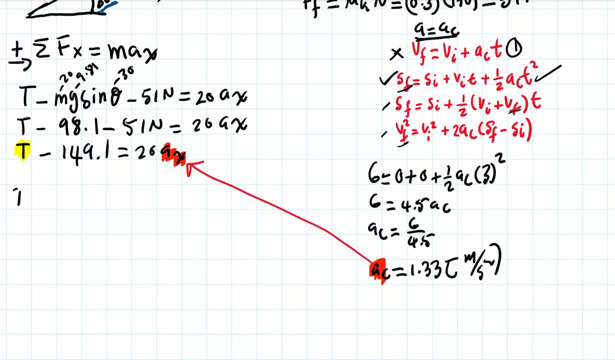 so tension. so what we will do is it will be minus 149.1, equal to 20 times 1.33. you know what we can simplify this? so it will be T and this will move to the other side of the equation. it will be: